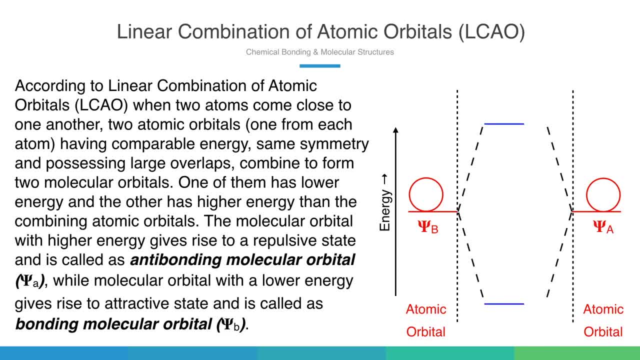 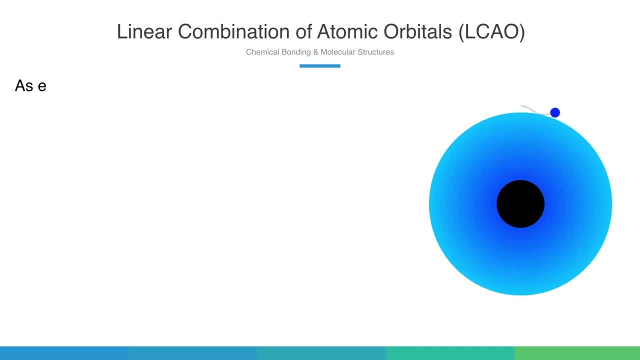 So, as you can see in the diagram, bonding molecular orbital tend to decrease the energy of the molecule and it increases its stability, while the anti-bonding molecular orbital increases energy and decreases stability. As electrons have dual nature of particle and wave, they can be considered as moving. 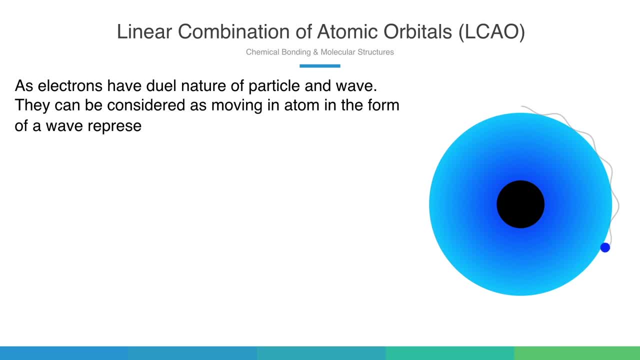 in atom in the form of a wave represented as psi. Let us consider: psi A is a particle, Psi A is a wave function of electron of atom A and psi B is wave function of electron of atom B. Therefore, wave function of bonding molecular orbital will be given by psi bonding. 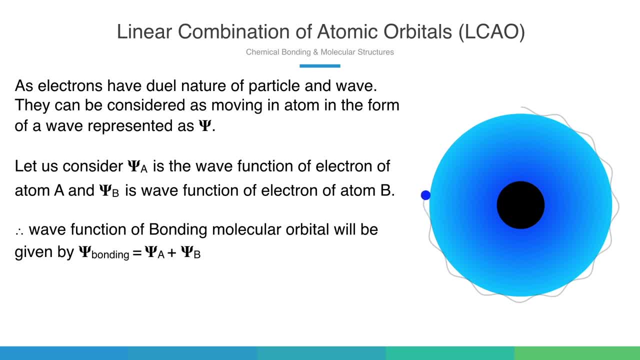 is equal to psi A plus psi B. It is the combination of two waves of two electrons of atoms, A and B, And wave function of anti-bonding molecular orbital will be given as psi anti-bonding, which is equal to psi A plus psi B. 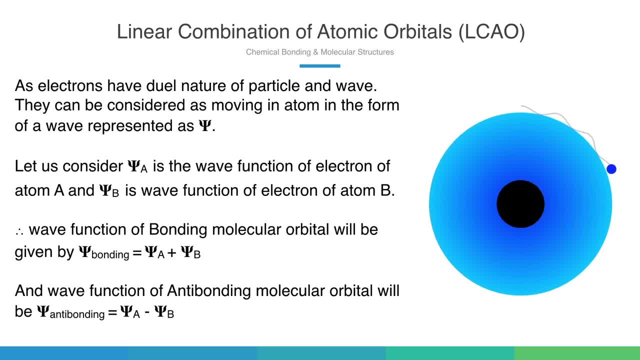 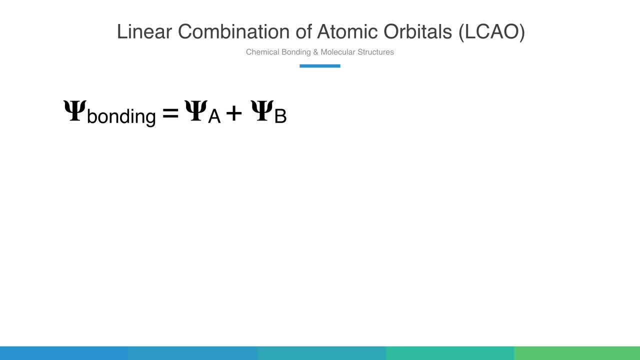 So it is the subtraction of waves A and B. A wave generally has a crest and a trough. When crest of one wave combines with crest of other wave, the amplitude of the resulting wave increases. The electron wave above the imaginary horizontal line is given a positive sign, while that 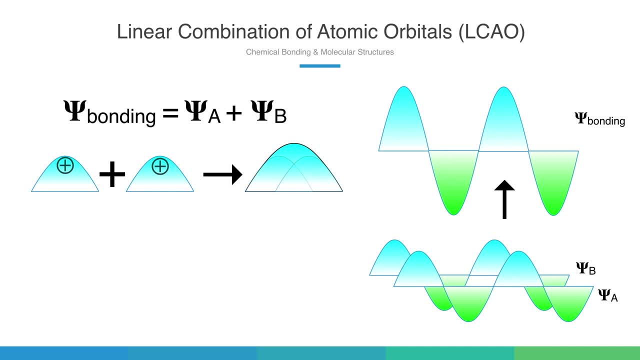 below is negative. In this case both the electron wave are on the same side. positive, That is the sign of the two wave functions are same. Such wave functions are regarded as they are in the same phase. When combine they give rise to larger resultant wave or molecular orbitals. 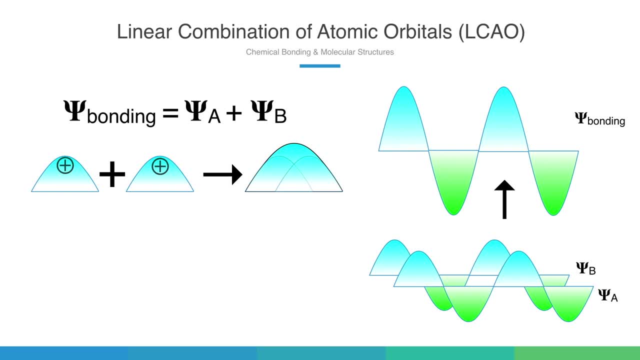 Such molecular orbital is called bonding molecular orbital. In this molecular orbital the region between the two nuclei is high electron density region, while the corners are low electron density regions. TIONAL RE interview. CATAR, ASP, cela 0 pup in the opposite direction. That means the crust of the one wave combines with the trough. 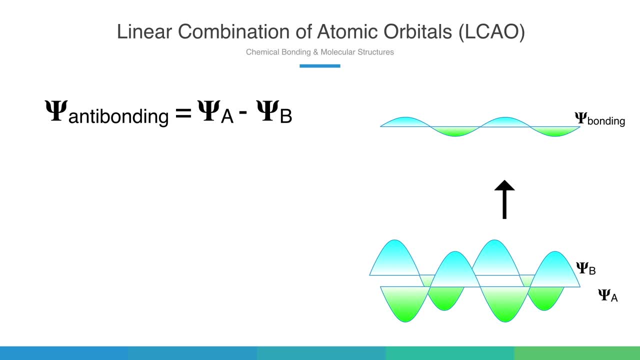 of the other wave. In this case both the amplitudes gets cancelled, as the waves are in out of phase position. We can also say that positive part of one wave combine with the negative part of the other wave, So they cancel each other. So in this case the probability